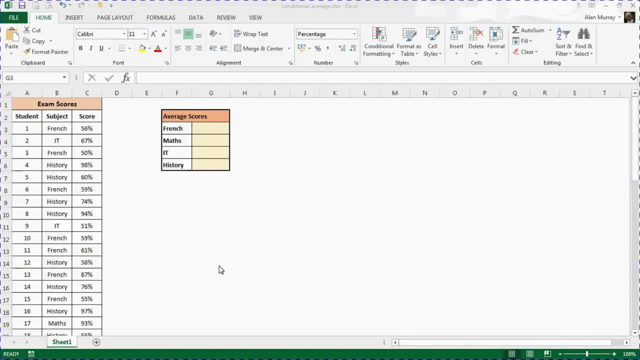 Hello and welcome to this video tutorial by ComputerGagacom, and in this video we want to look at how to create a conditional average. So our goal is to find the average for the various subjects within this list. So the average is conditional. We want to find the average if it's. 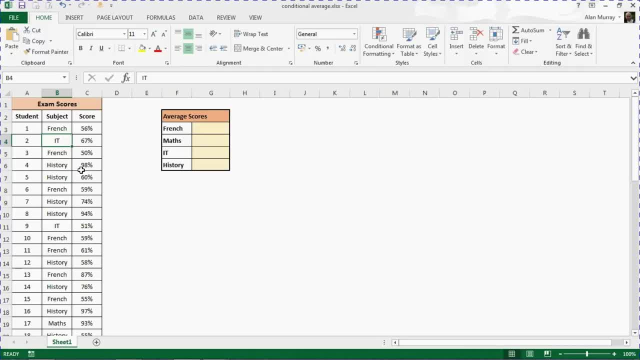 the French subject and if it's IT and so on, And we're going to put this information in this little kind of summary table we have on the right, starting with G3 and the French scores: French exam scores. Let me zoom this spreadsheet in so we can see the formulas are right a bit easier. 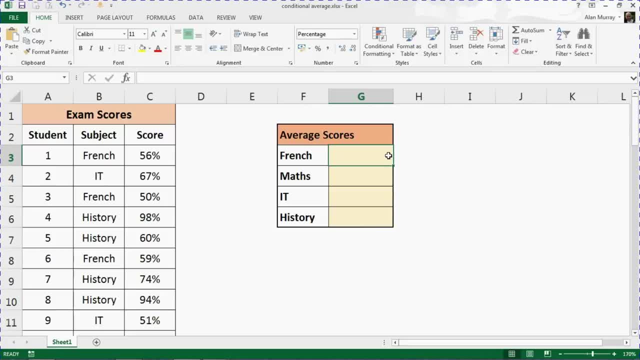 and get started, And we are going to use a function called average, if So, average if it is that subject, And we have three arguments or three questions to tackle. Question one is the range that we're testing, In this case what subject, and for us that will. 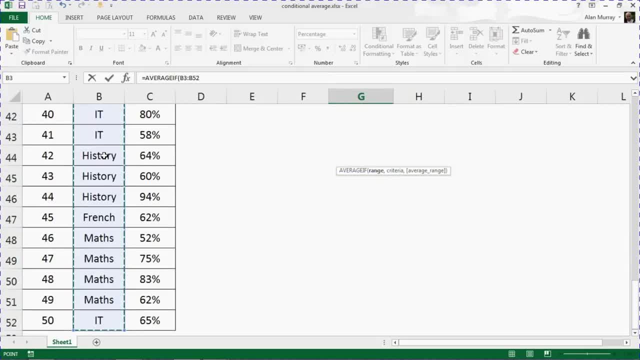 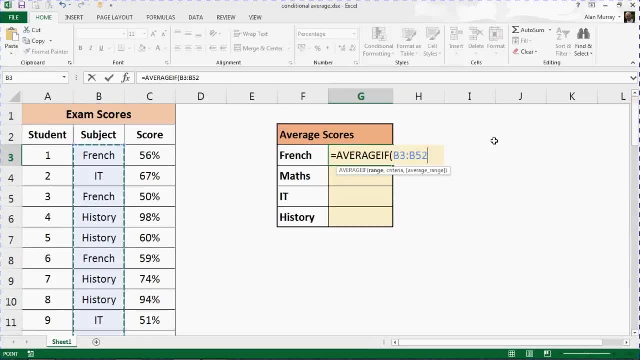 be B3 to B52.. Using my ctrl, shift and down keys there to quickly select that. Now, when we are finished with this formula, I'm going to copy it to the maths, IT and history subjects as well. So I'm going to want to fix that range so it doesn't change when I copy this. 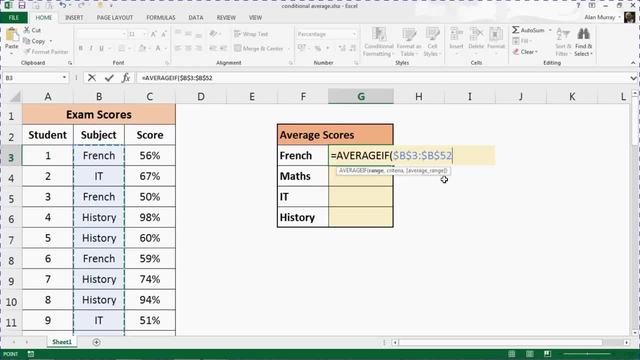 formula. I did that by pressing the F4 key- the function key, F4 there- and dollar signs can alternatively just be typed in, though, Or you could just change it for the others and not worry about the dollar signs, But I'm doing that so that the range does not move when I move the formula or copy the formula. 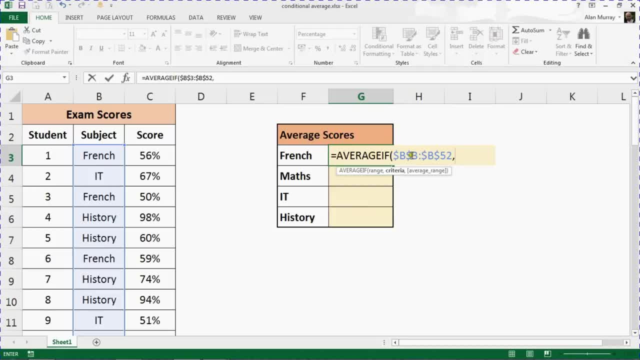 A comma after that, so it asks for the criteria we are looking for within that range, And that is F3.. I'm going to refer to the cell that contains the name and subject that we're looking for, And I won't use dollar signs there, because when I copy the formula down I want the.